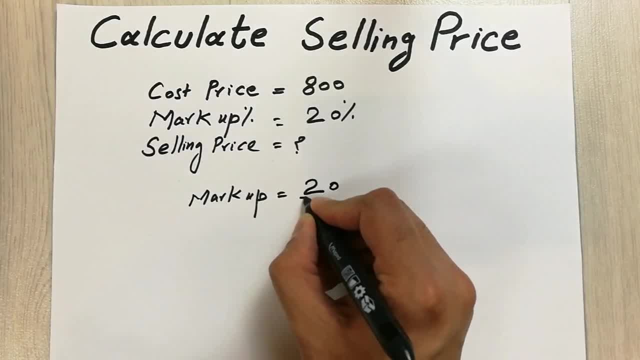 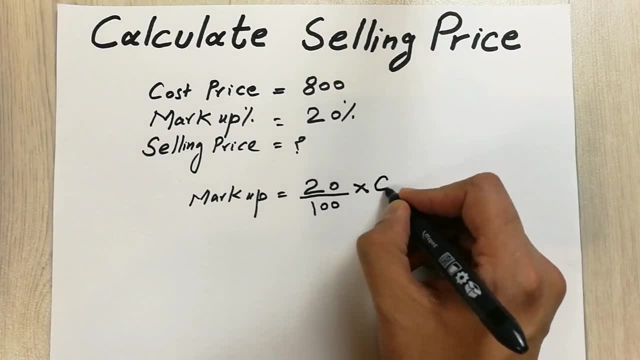 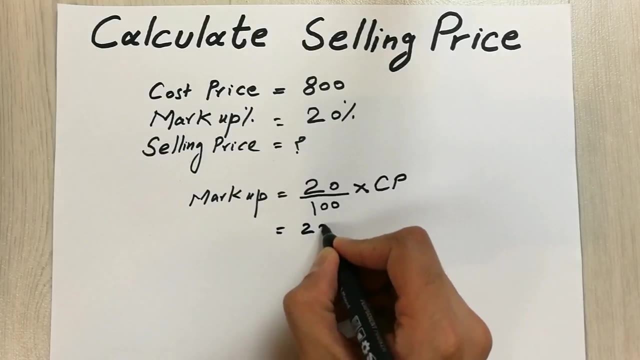 20 percent. we have to divide it with 100, okay, and then we have to multiply it with the cost price, okay. so our cost price here is 800, okay, so what we're going to do is we divide 20 with 100 and we multiply it with 800, which is the cost price. okay, so these two zeros, they will cut it. 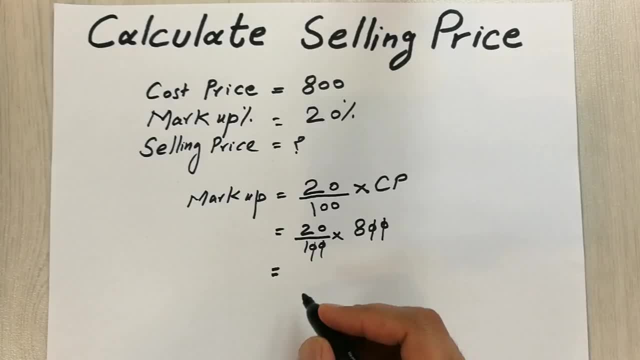 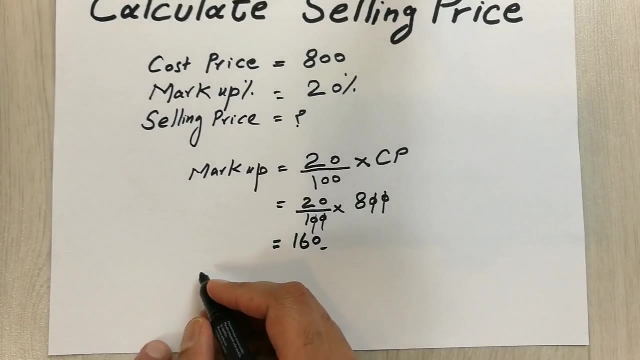 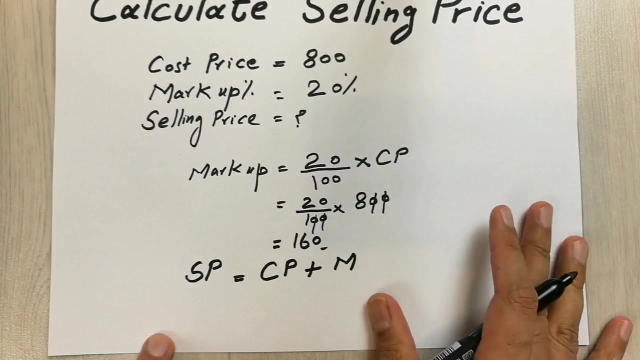 from here and then 20 multiplied by 8, the answer will be 160. okay, guys, so this 160 is our amount of the markup. okay, in the next step we have to simply put the formula to calculate the selling price, or SP. so the formula is cost price plus this markup. okay, so now we will put the value, the 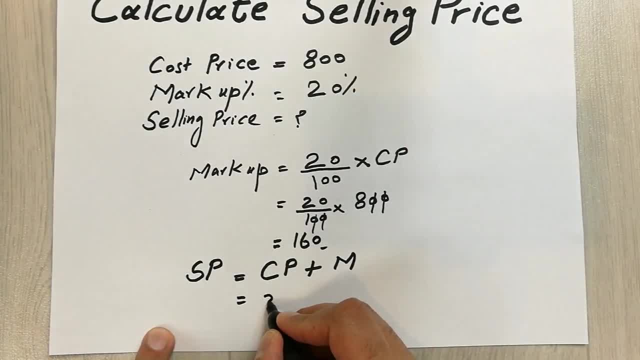 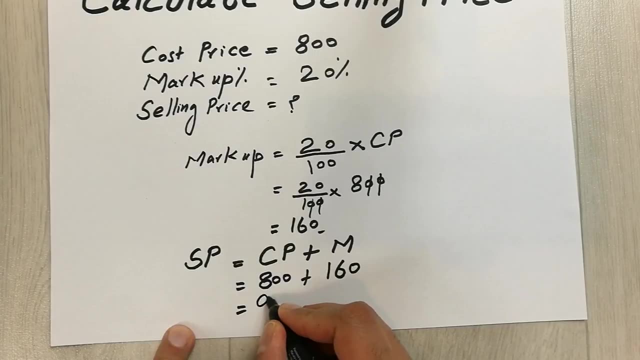 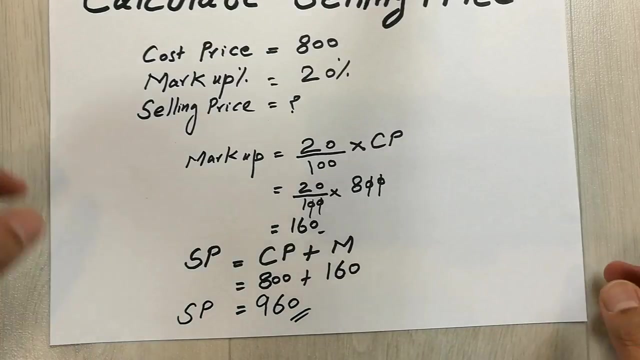 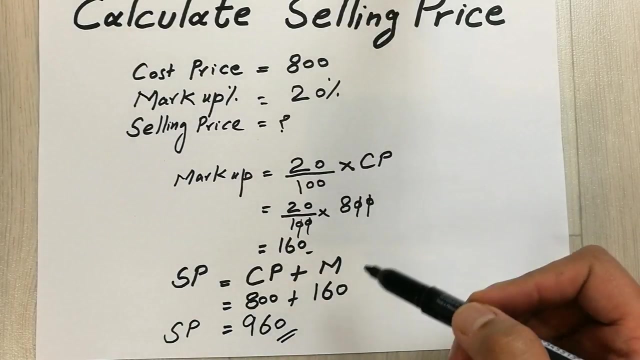 cost price is here, which is 800, okay, plus this markup we already calculated- which is 160. so our cost and 60, so, guys, this is our selling price. so this is how you can calculate the selling price in the two steps. okay, the first step: you find the amount of the markup. in the next step, you just 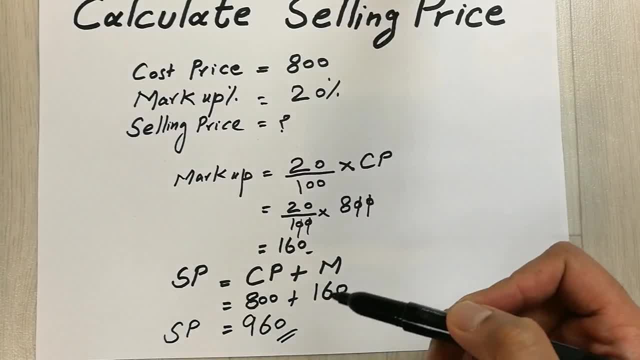 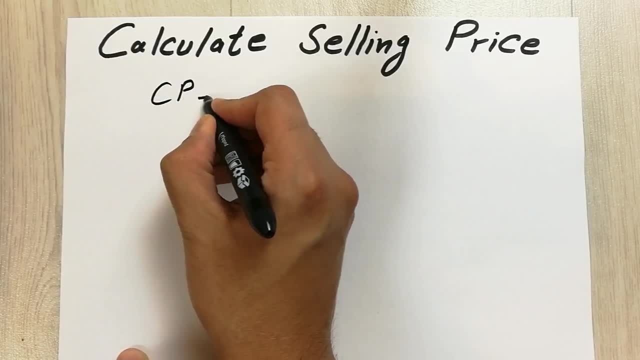 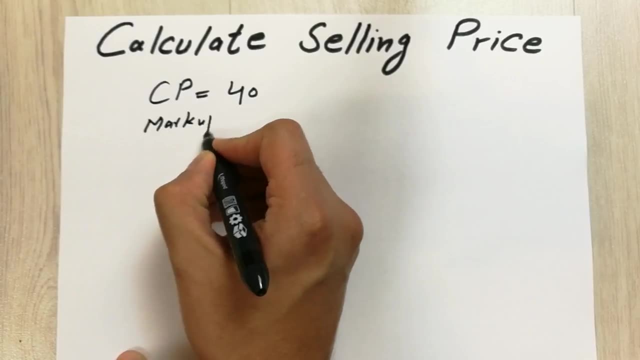 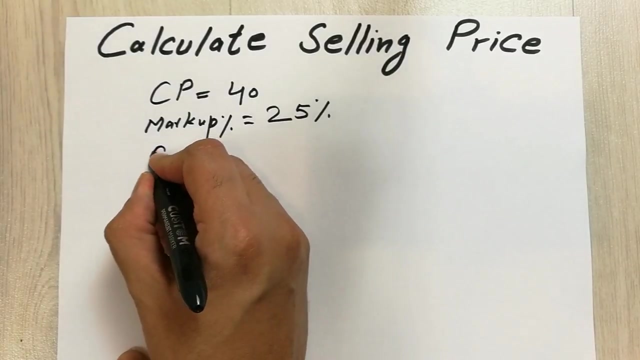 simply put the formula and put the values and you will get the answer. i will show you with one more example. let's say you have a product and the cost of the product is 40 dollars or rupees and the markup percentage is, uh, 25 percent. okay, guys, and now you want to calculate the selling price. 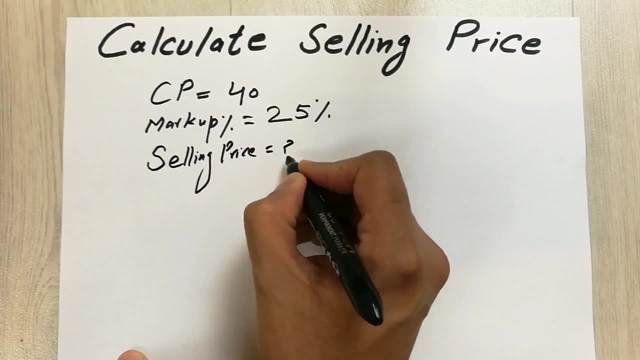 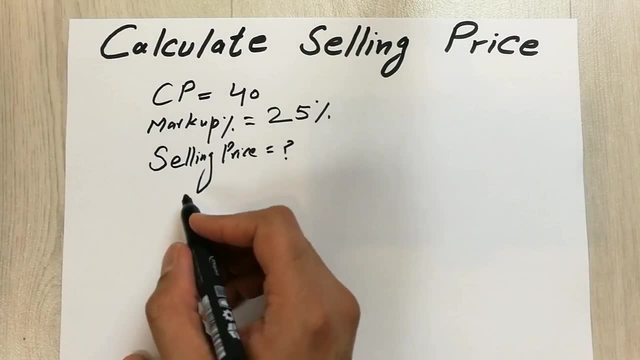 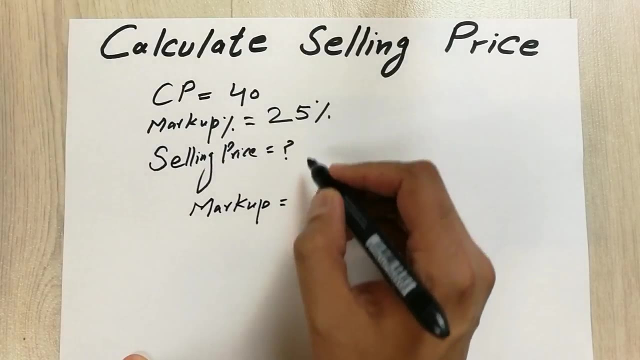 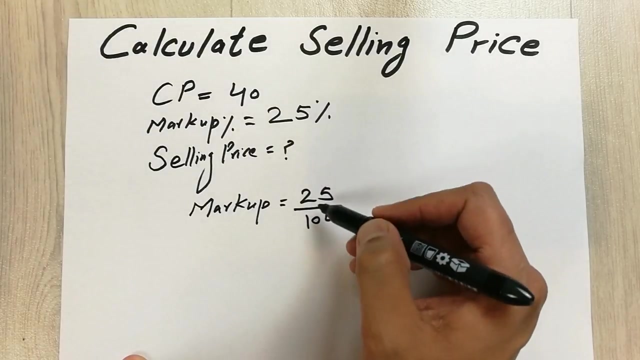 okay, okay. so first of all, what we're going to do is we will find out the amount of this markup percentage. okay, so, to find out the markup amount of markup, we have to divide this 25 with 100, because you know there is a percent. so it means 25 divided with 100, and then we